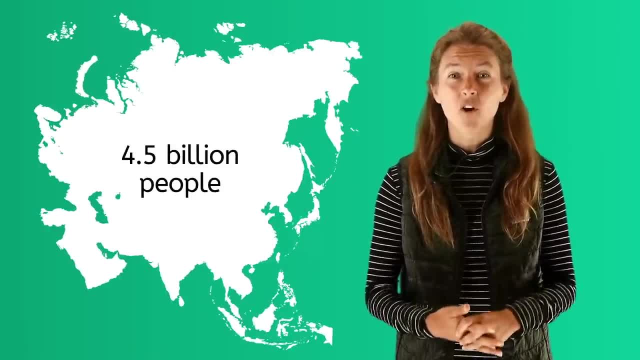 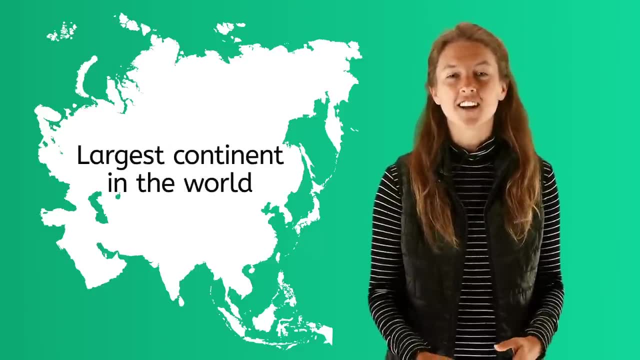 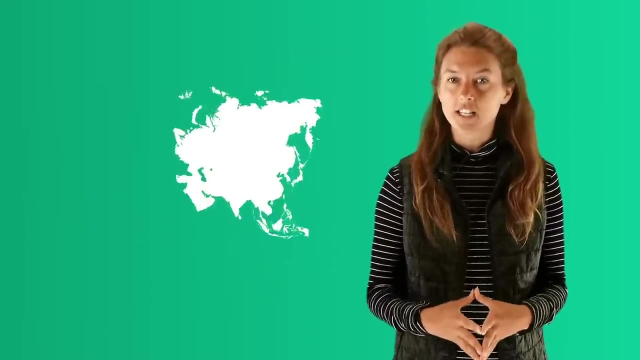 Asia is the most populated continent in the world, With over four and a half billion people living in it. Yes, billion. It is also the largest continent in the world. Asia is located mostly in the northern and eastern hemispheres, and it is surrounded by the Arctic Ocean to the north, the Pacific Ocean to the east. 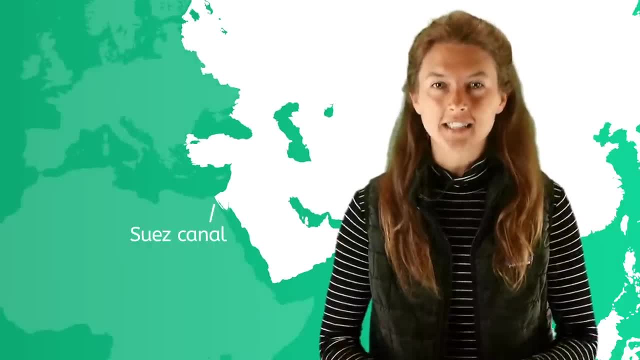 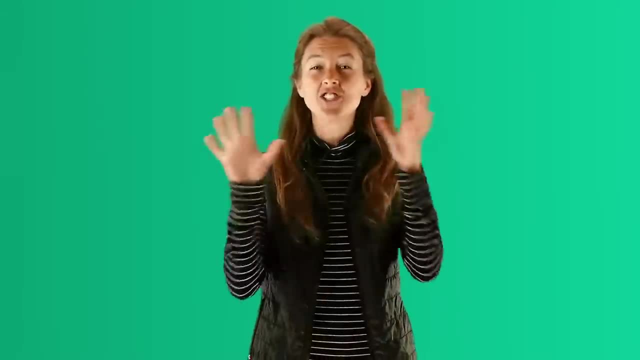 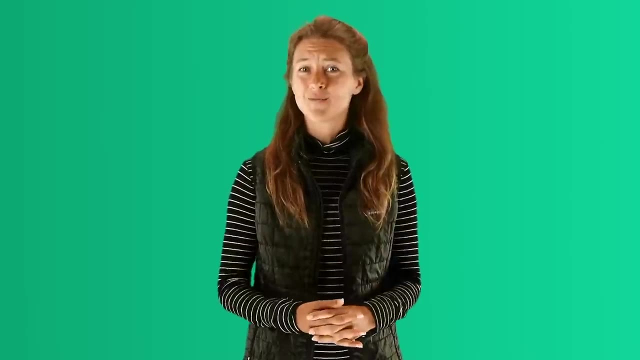 and the Indian Ocean. to the south, The Suez Canal separates Asia from Africa, and the Mediterranean Sea and the Black Sea separates it from Europe. There are hundreds of continents in the world. India alone has 30 official languages. The most common languages spoken in Asia are English. 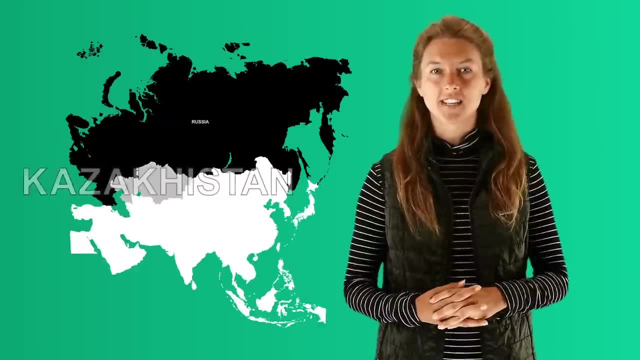 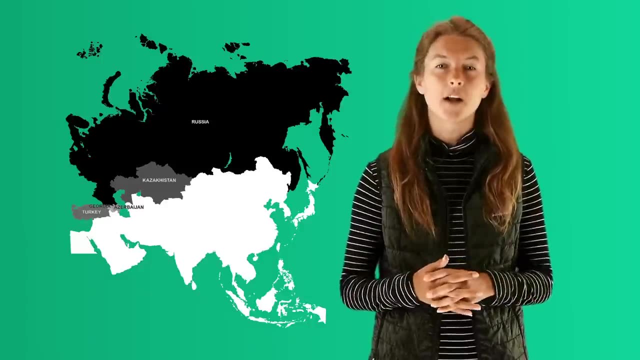 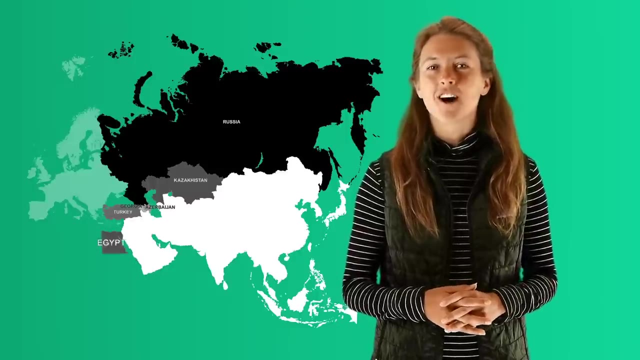 Arabic and Mandarin, Chinese, Russia, Kazakhstan, Azerbaijan, Georgia and Turkey are transcontinental countries, which means they are part of more than one continent. In this case, they are both in Europe and Asia. Egypt is also a transcontinental continent. 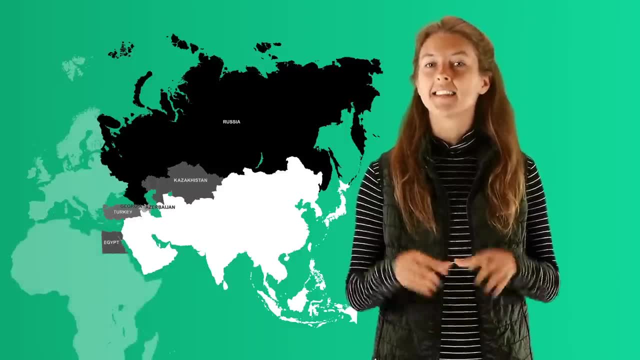 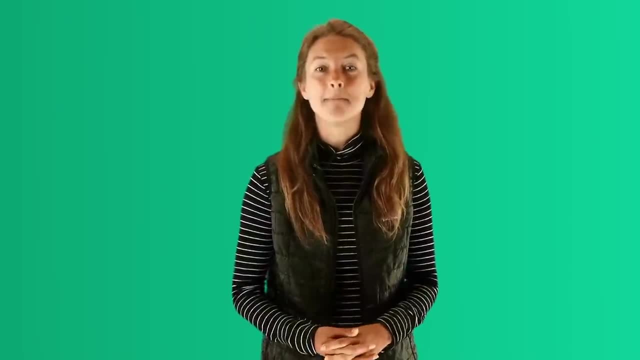 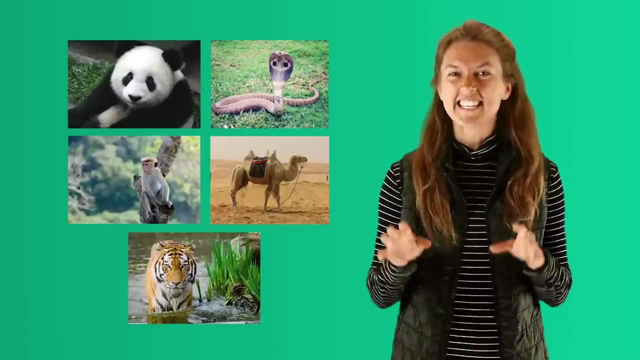 The Middle East is a country found in both the northeast corner of Africa and the southwest corner of Asia. also known as the Middle East, Asia is home to some amazing animals, including the panda- my favorite cobra- macaque, the camel and the tiger. 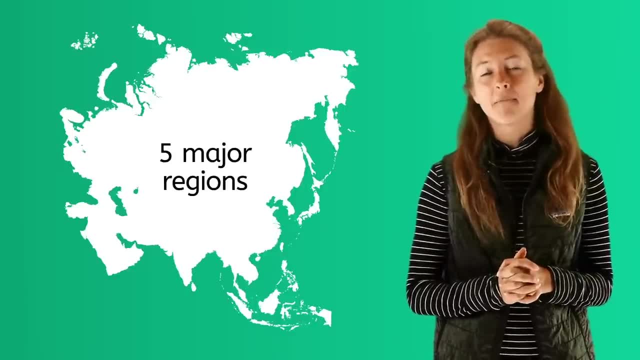 There are 48 countries in Asia and five major regions, So we have Southeast Asia, East Asia, South Asia, Southwest Asia and the Middle East. There are 48 countries in Asia and five major regions, So we have Southeast Asia, East Asia, South Asia, Southwest Asia and the Middle East. 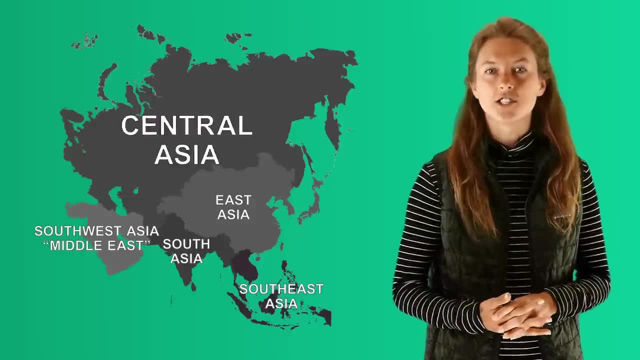 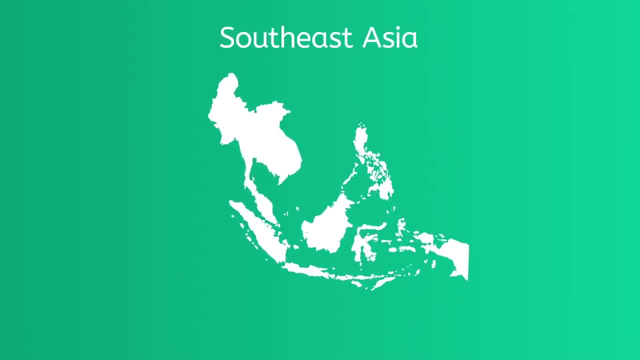 There are 42 countries in Asia and six major regions, Which is commonly referred to as the Middle East and Central Asia. Let's break down each region. Southeast Asia has a very wet climate, with a monsoon season or the season with rain for. 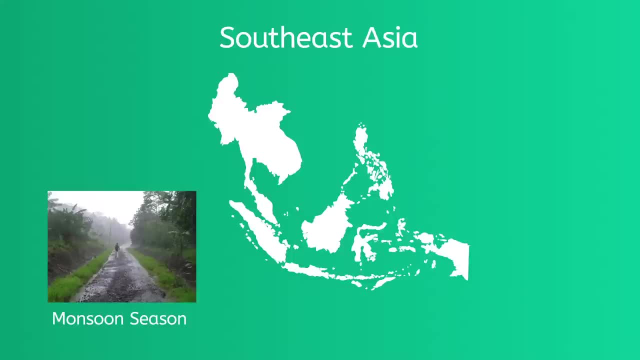 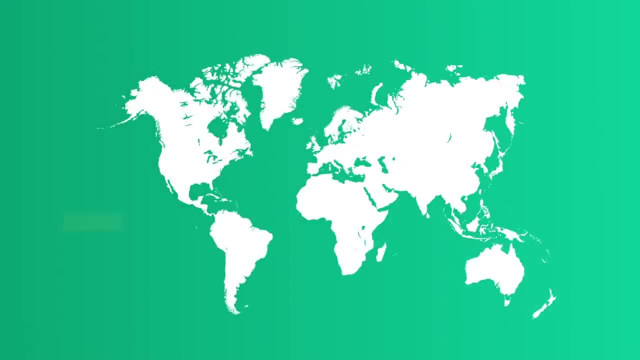 many, many months, typically between May and September. Imagine that, oh, This part of Asia is covered in rainforests. Also, the equator runs through Southeast Asia. The equator is hot. In fact, they make up about 15% of the space on the tip of their heads. 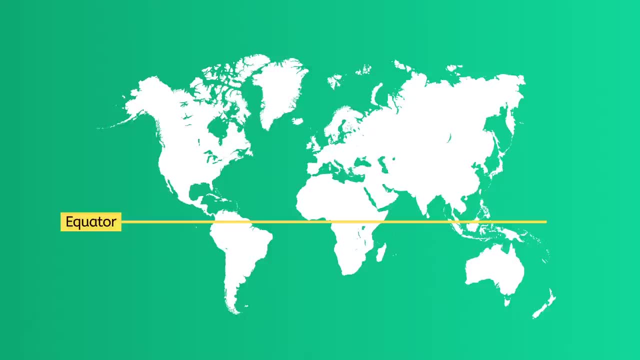 The equator sits on the defensive elements of East and West, an imaginary line around the earth splitting the earth into the northern and southern hemisphere. near the equator, the temperature is a lot hotter and more humid than other parts of the earth, making it feel like summer all year round. you can find these. 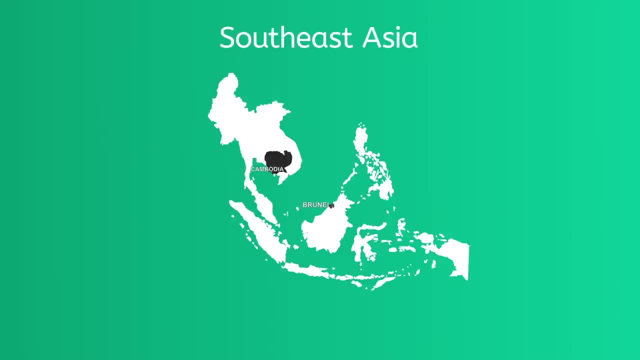 countries in this region: Brunei, Cambodia, where we can find the largest known temple on earth. in Indonesia, the country with 15 000 islands, Laos, Malaysia and Myanmar, which was once Burma, and tea is the most popular drink in this country. who doesn't love tea? then we find 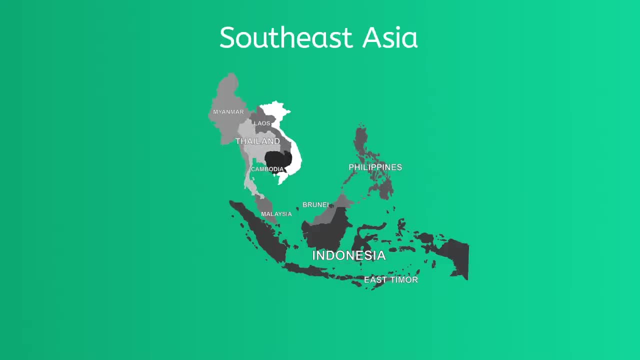 the Philippines, East Timor, Thailand, where there are over 30,000 Buddhist temples. Singapore, which is both a city and a country, and Brunei, Cambodia, where there are over 30,000 Buddhist temples. and Brunei, Thailand, where there are over 30,000 Buddhist temples. 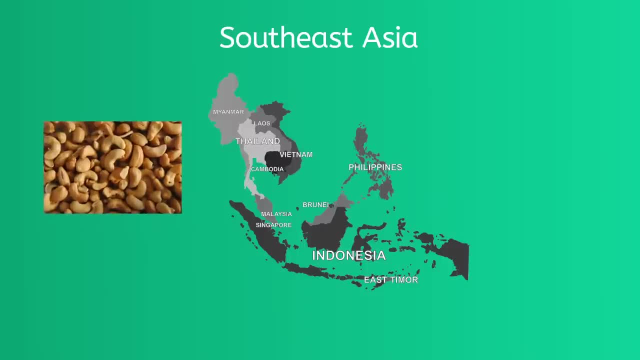 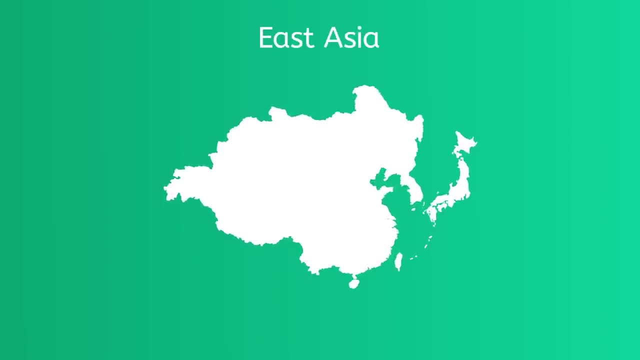 and Brunei. Thailand, where there are over 30,000 Buddhist temples, And finally Vietnam, the country from which the world gets most of its cashew nuts and black pepper. In East Asia, the climate is subtropical, meaning they experience hot, humid summers. 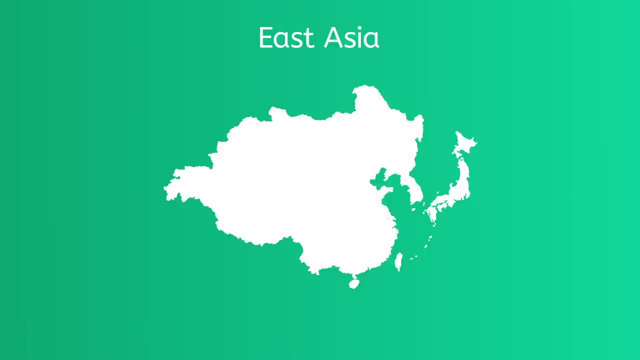 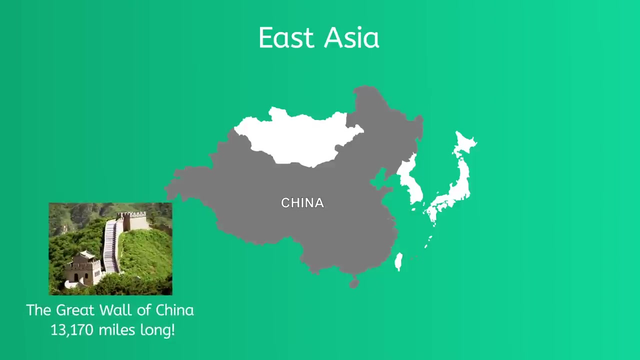 and mild to chilly winters. Let's look at the countries found in East Asia: China, which has been the most populous country in the world for many centuries, but is now being overtaken by India. It is also where you can find the Great Wall of China, the longest structure ever built. 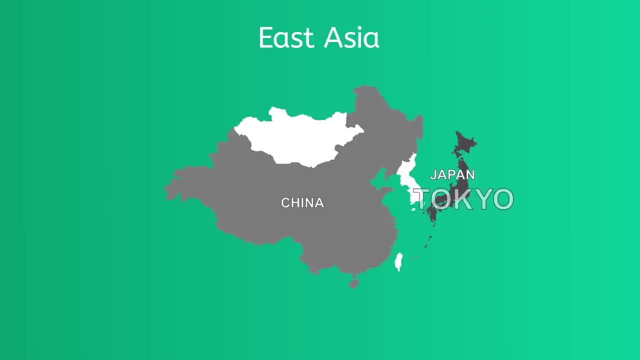 by hand. Then there's Japan, with Tokyo as its capital. The megacity of Tokyo, Yokohama, is the largest of the world's megacities. Japan is famous for the animation styles of anime and manga. Mongolia, which is a country considered to be landlocked, meaning it does not have access. 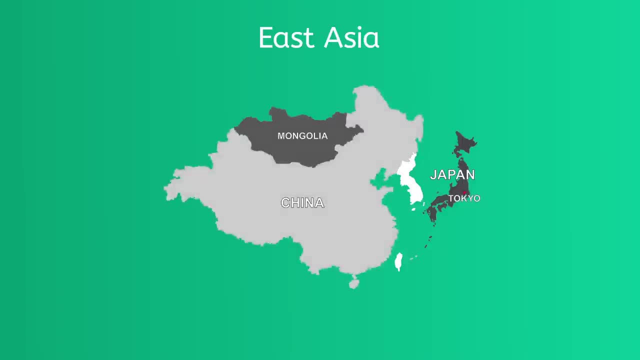 to an ocean. This country is located within China and Asia. In this region we have the countries of North and South Korea. Taiwan is also found in East Asia. Both Chinese government in Beijing and the government of Taiwan say that there is only one, China, and Taiwan is part of it. 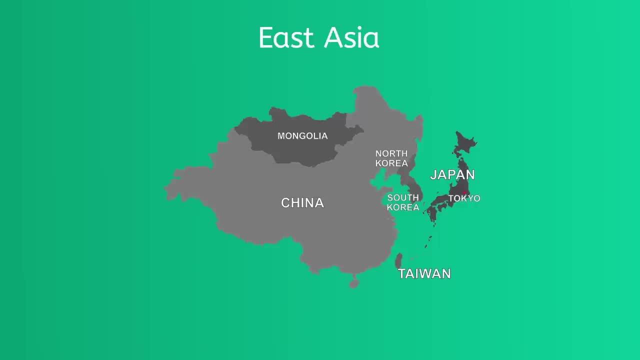 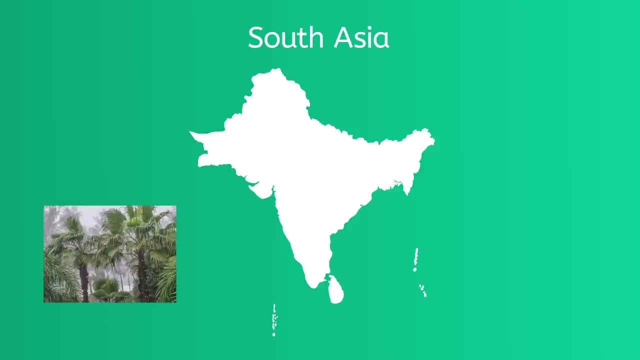 But it has been governed independently since the 1950s. Moving on to South Asia, we find a variety of climates, from hot tropical monsoon in the south To hot but cooler in the north. The countries found in South Asia include Bangladesh, Bhutan and India. 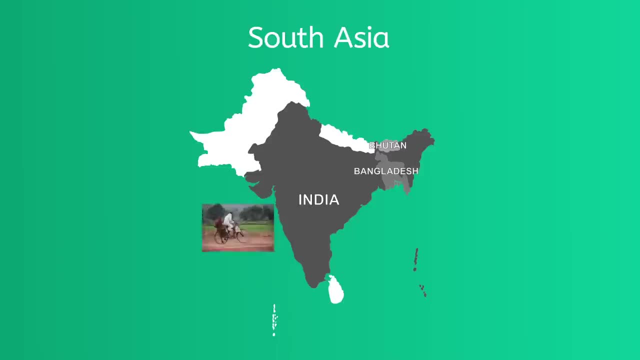 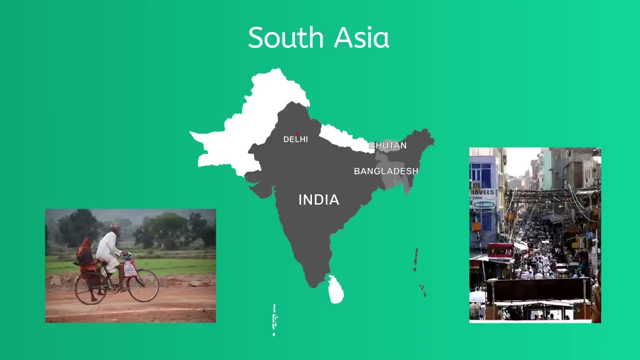 A popular travel destination in this region, where many of the locals get around by bicycle. It is also home to the city of Delhi, one of the world's largest megacities, because it suffers from overpopulation. The population of India has been growing fast for many years and it is now becoming the 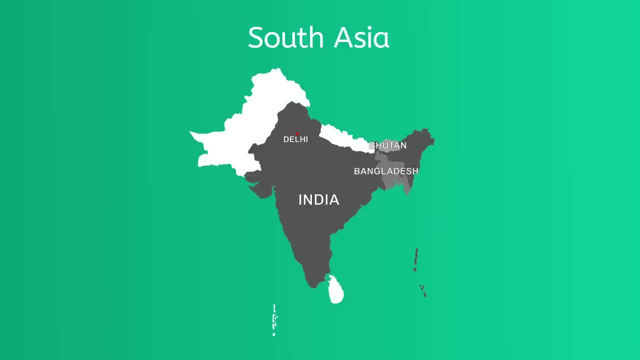 most populous country in the world. Continuing in this region, we have the Maldives, which is the smallest country in Asia, both by size and population. It is also a popular vacation spot famous for its beaches. Nepal, where Mount Everest is the highest mountain on earth, is home to the city of. 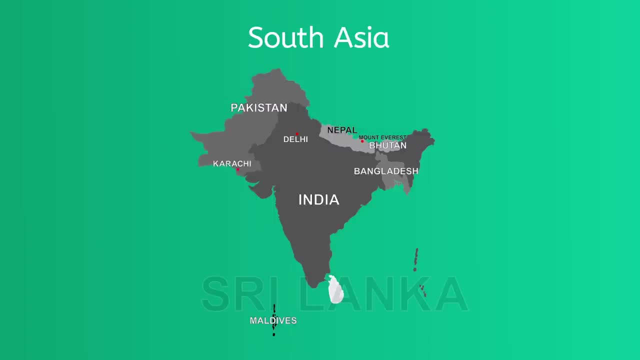 Karachi, Another one of the world's largest megacities, and Sri Lanka formerly named Ceylon, has the world's largest sought-after and expensive blue sea. The Maldives, which is the largest mountain on earth, is home to the city of Karachi. 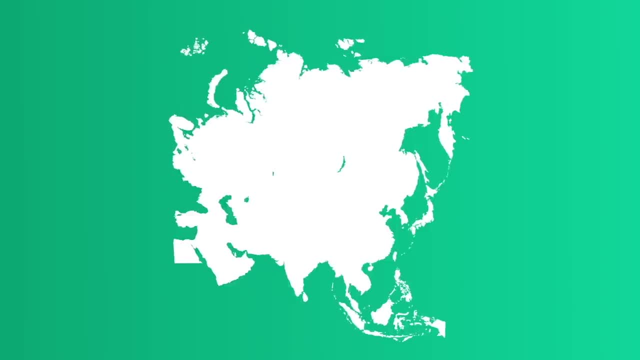 one of the world's largest megacities and Sri Lanka formerly named Ceylon, has the world's largest sought-after and expensive blue sea. The Maldives, which is the highest mountain on earth, is home to the city of Karachi. 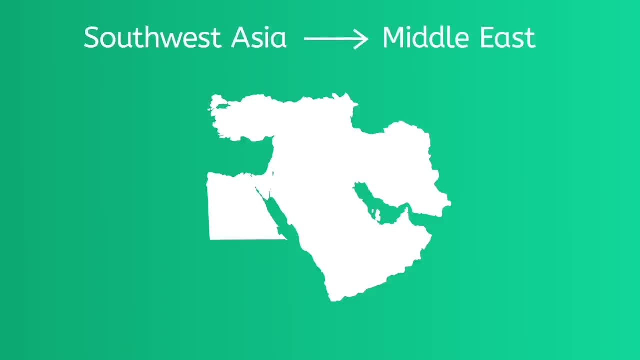 and Sri Lanka, currently named Ceylon, has the world's largest sought-after and expensive blue sea. The Maldives, which is the highest mountain on earth, is home to the city of Karachi, one of the world's largest sought-after and expensive blue sea. 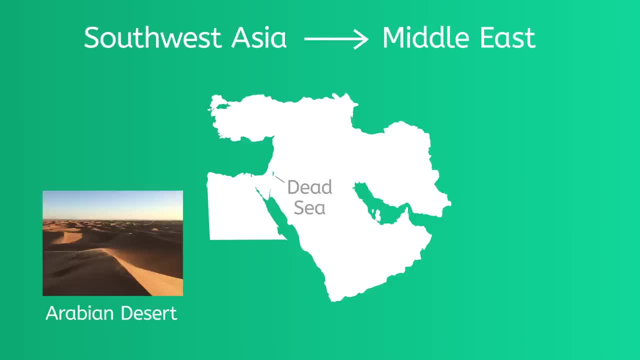 This region is also where the lowest point on earth, the Dead Sea, is located. Much of the world's oil comes from the Middle East. The countries that make up the Middle East are Azerbaijan, Guinea, Afghanistan and Bahrain. Egypt. Georgia- Be careful don't confuse this country with the state of Georgia in the USA. 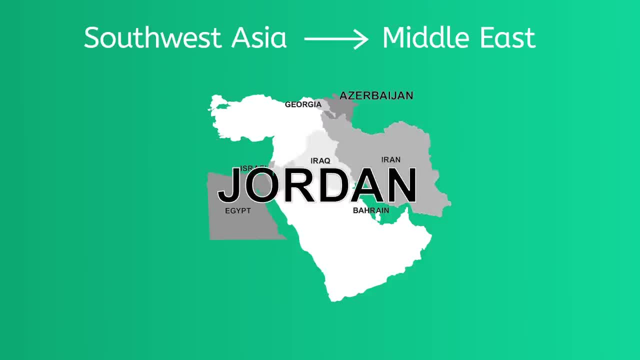 Iraq, Iran, Israel, Jordan, Kuwait, Lebanon, Oman, which is a country known as an important sea turtle breeding site. that includes the green sea turtle, the leatherback sea turtle and the loggerhead sea turtle. Then we're on to Palestine, a country that is not recognized by the US.